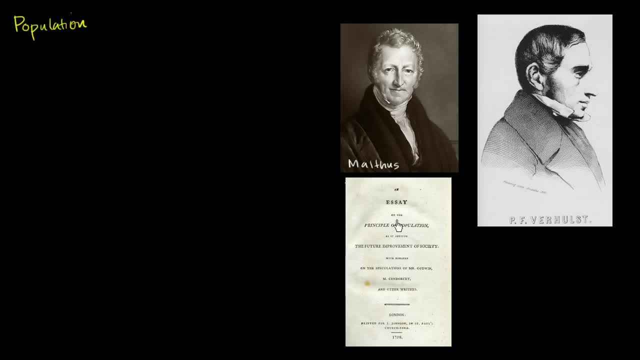 and then they would go crashing below the limit and you would kind of oscillate right around the limit through these catastrophes. As you can tell, Malthus was a fairly optimistic guy, But let's go through a little bit of the math. 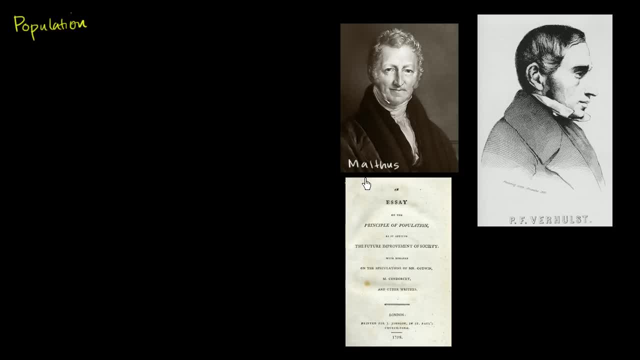 and a little bit of the differential equations. Although it's not too, these aren't overly hairy differential equations to think about population. So the first way to think about population, and I'll express it as a differential equation, So let's just actually let me just set some variables here. 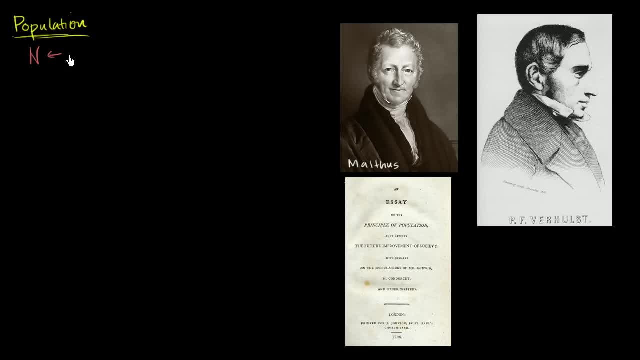 Let's say that N is our population, So that's our population, And we are going to assume that N is a function of T. So N as a function of T is what we're going to be thinking about in this and, frankly, the next series of videos. 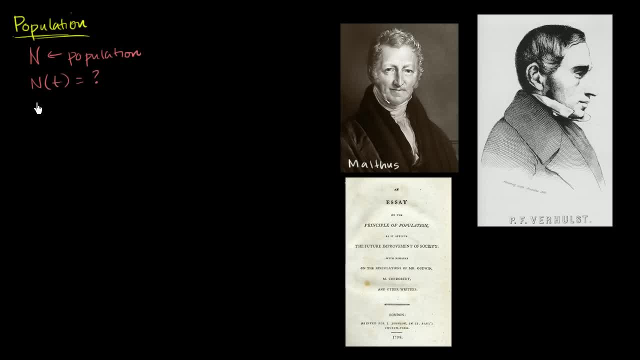 So one way to think about how to model this is just to say, well, how does what is the rate of change of population with respect to time? How does that relate to things? And so we could say, okay, well, what is the rate of change of population? 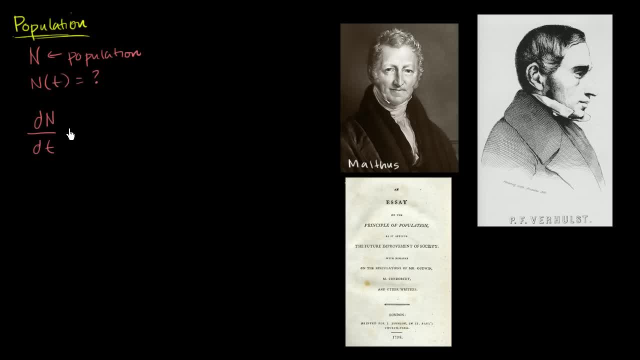 with respect to time. So D capital, N DT. Well, one way to think about it is it's going to be proportional to the population. So you could say, well, maybe this is going to be some proportionality: constant times the population, times the population itself. And this makes sense. If the population is smaller, then you're not going to have as much as much change per unit time as if the population is larger. The larger the population, the more it's going to grow in a particular unit of time. 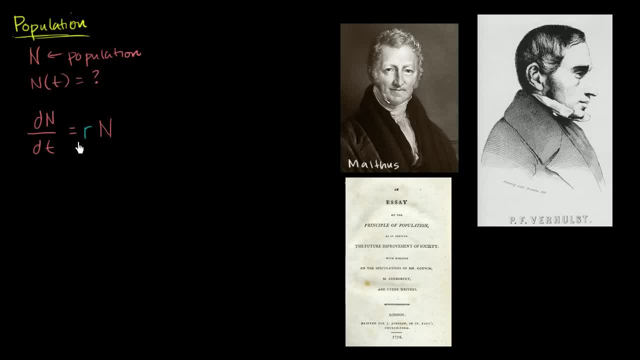 And actually this is actually a very, a fairly simple to solve differential equation. You might have done it before. I encourage you to pause this video if you feel inspired to do so, But I'll solve it right here and you'll see that we get an exponential. 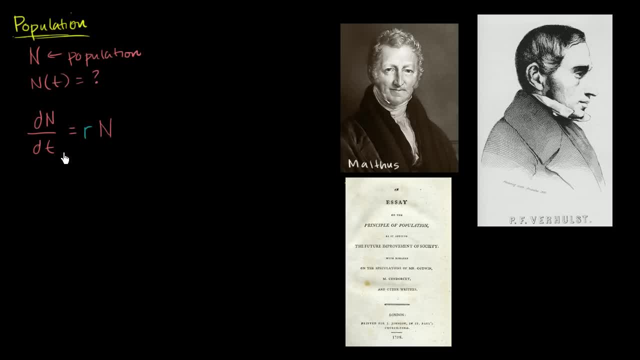 we get an exponential function here for N. So let's do that, So let's solve this, and we'll essentially separate the variables, separate the N from the T's, although we don't- we only see a DT here, but I'll do that in a second. 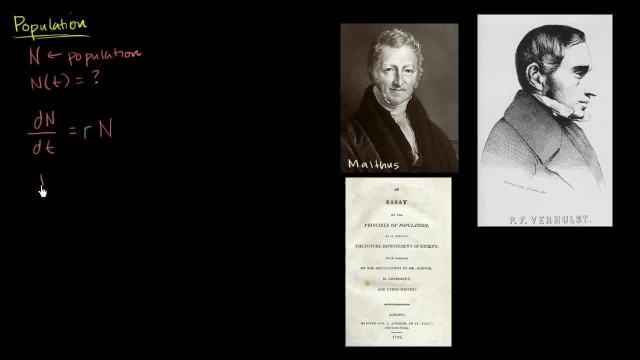 So if I divide both sides by N, I get one over N. And if I multiply both sides by DT, if you kind of think about the DT as something that you can multiply, So I'm going to multiply both sides, or I'm going to divide both sides by N. 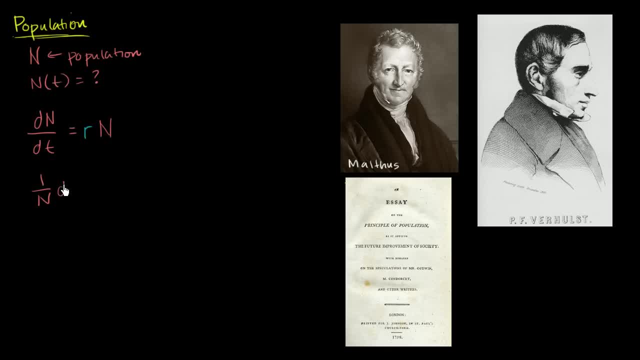 and multiply both sides by DT. So I'm going to get one over N DN on the left-hand side And on the right-hand side I'm going to get R times, DT. R times, R times, DT. Notice, I got the DT onto the right-hand side. 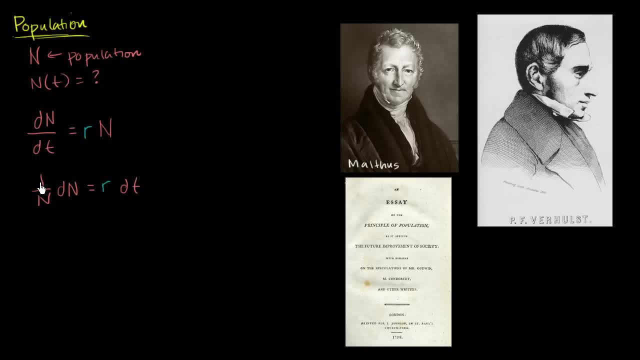 by multiplying both sides of that And then I divided both sides by N and I got the one over N right over here. Now what we can do is we can take. we can take the antiderivative of both sides. We can take the antiderivative of both sides. 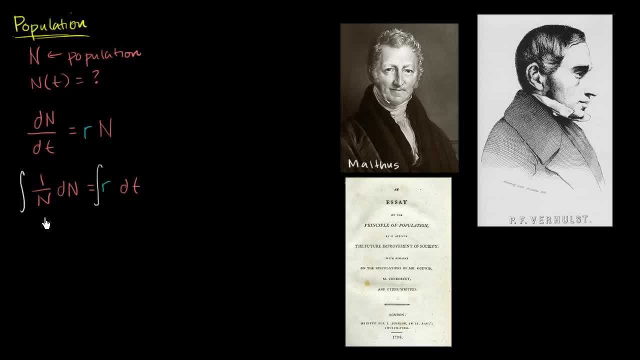 And what do we get on the left-hand side? Well, this is just going to be the natural log. this is just going to be the natural log of the absolute value of our population And, actually, if we assume that the population is always going to be non-zero, 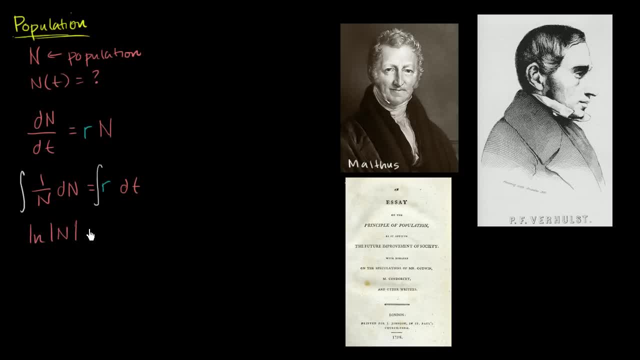 then we can actually take this, this absolute value, off. but I'll do that in a second, And that's going to be equal to R R times T, R times T, And then we could have added a constant here, but I'm just going to do it on one side. 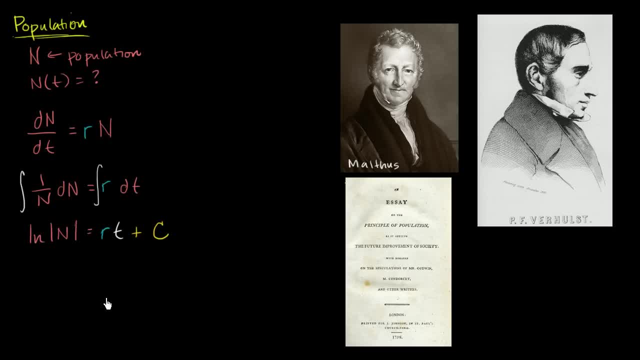 So it's R times T plus R times T plus C. And now if we actually want to solve for N we could take, we could take. if this is equal to this, then E to this power should be the same as E to this power. 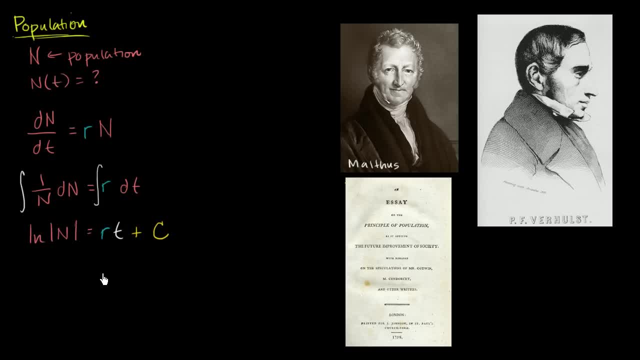 Another way of thinking about it. E, the natural log of the absolute value of N, is equal to this is another way of saying that E to this is going to be equal to that. Well, actually, let me just do it this way. Let me just take 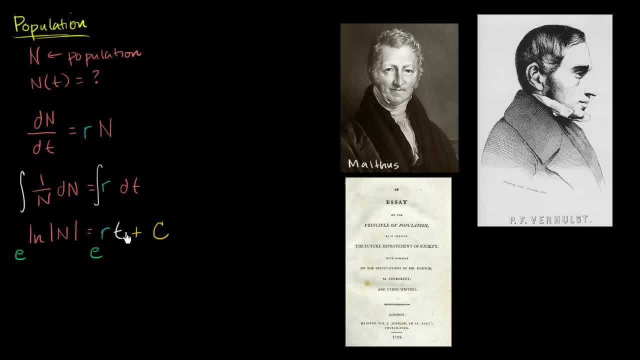 let me just take E to both, to both to this power and to that power. If that's equal to that, then E to that power should be the same as E to that power, And so we're going to be left with E. 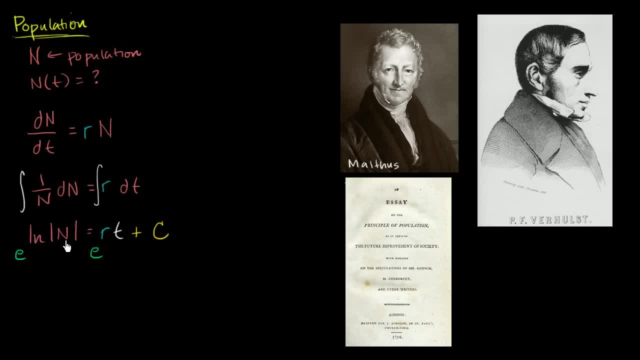 the E to the natural log, E to the natural log of the absolute value of N. that's going to give you the absolute value of N. Let's just assume, assume N positive Assume, let's just assume population is greater than zero. 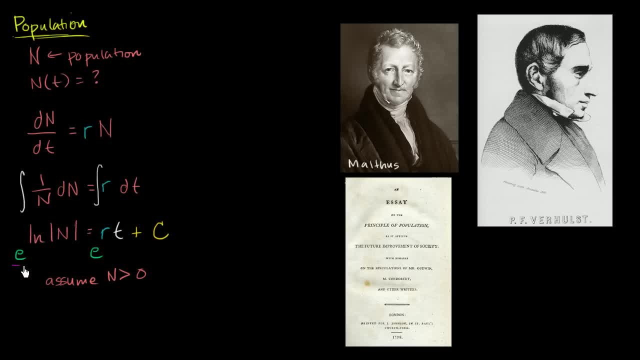 And so then we could this left hand side, this left hand side right over here, we'll just simplify to N- And then our right hand side. it's going to be. well, it could be E to the RT plus C, or this is the same thing. 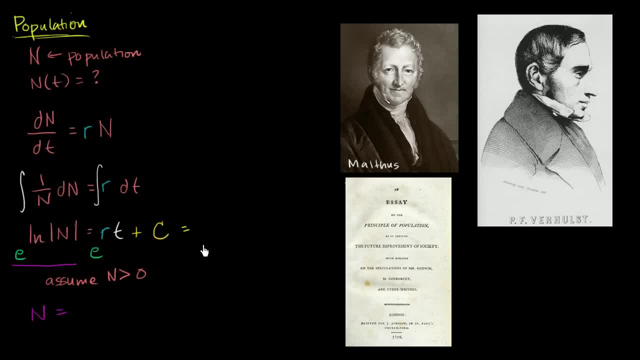 this is this thing right over here is the same thing as E to the RT, E to the R times, T times. actually, let me do that E in that same color: E to the RT times, E to the C times, E to the C right. 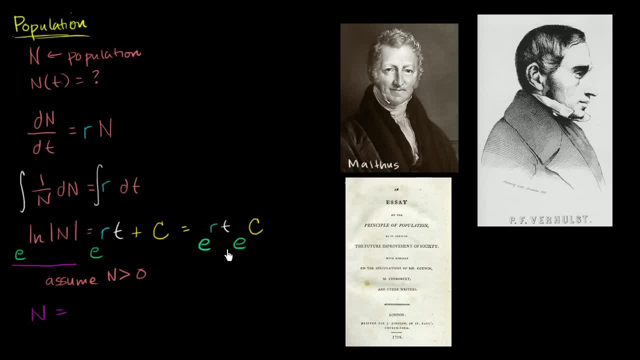 I'm just taking E to the sum of these two exponents. that's just going to be E to the RT times, E to the C, And if we want to, we could just say, hey, you know what? This is still just going to be some arbitrary constant. 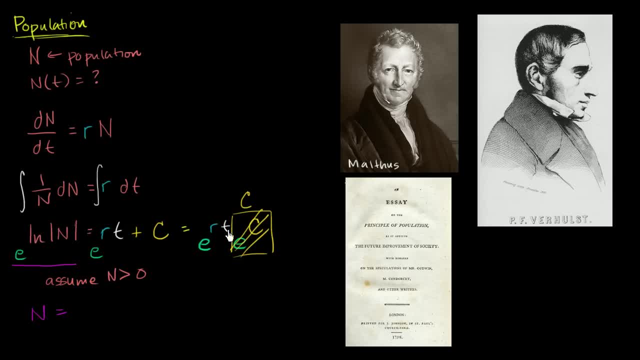 So actually, let's just call this, let's just call this C, So it's E to the RT, times C, or we could say C times, E to the RT, C times E, E to the R, E to the RT, And notice. 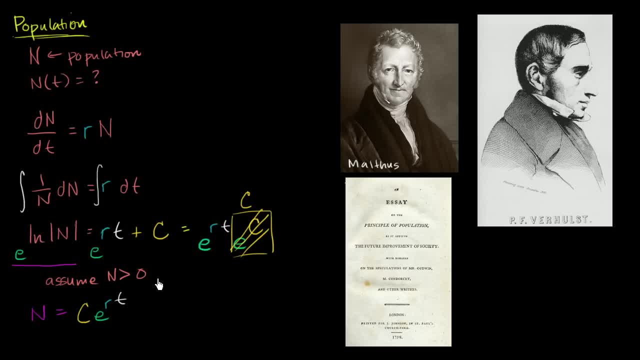 so we have solved the differential equation. We haven't gotten to this kind of less than optimistic reality of Malthus where we're limiting it. This is just hey, if we just assume population is going to the rate of change of population with respect to time. 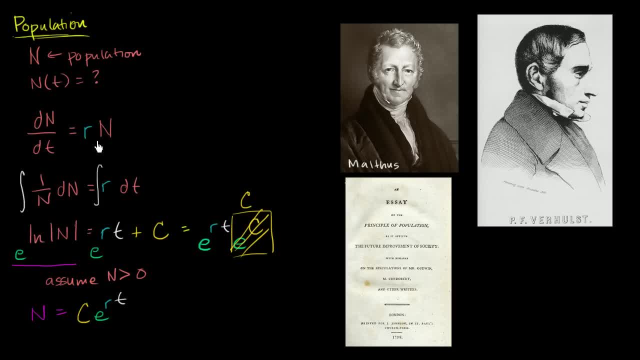 is going to be proportional to population. When we solve that differential equation, we get that population is a function of time. Actually, let me make it explicit that this is a function of time, So let me just move the N over a little bit. 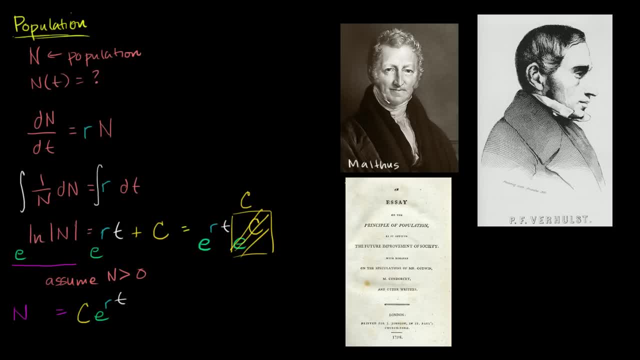 So let me write it this way: N of T is going to be equal to this. This was our solution to our differential, to this differential equation And, once again, this is just going to grow forever And if we know the initial conditions, 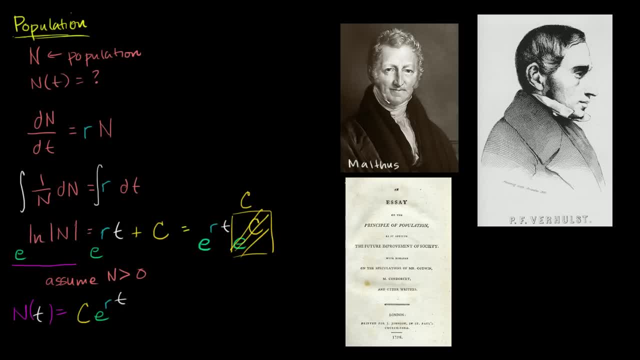 and so let's say that we knew that. N of zero. when time is equal to zero, let's just say that's N sub-naught. So what would C be? Well, N of zero is going to be equal to C times E, to the zero power. 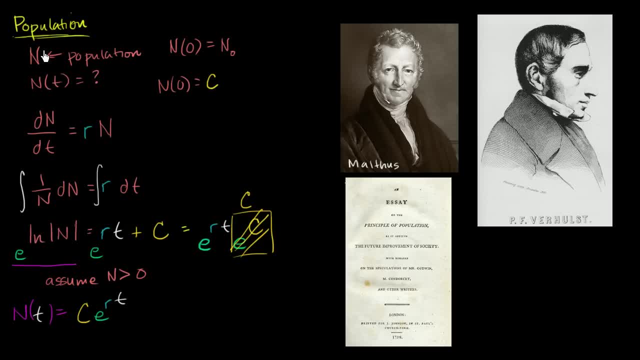 E to the zero power is just one, so it's just going to be equal to C. So C is equal to N sub-naught. So now we can even write it that the solution to this thing right over here is N as a function of T.